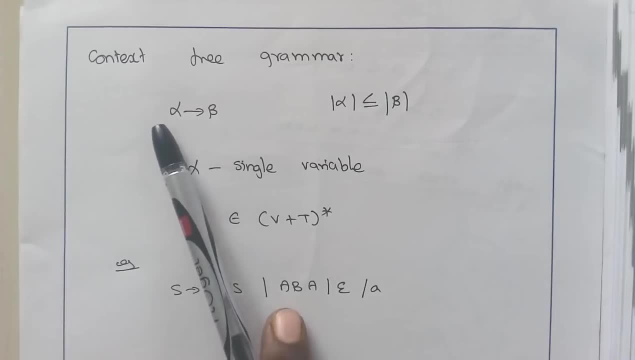 is called a production rule and there are some restriction in the rule. It is of the form alpha tends to beta and this length of alpha should be less than or equal to beta. and this alpha, it is always a single variable. So alpha, it should be a single variable. 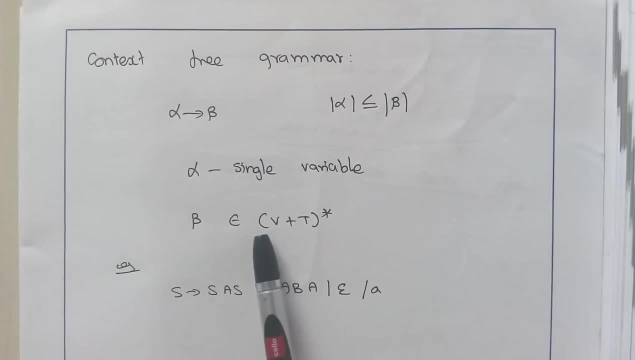 whereas beta it might be either a variable or a terminal or any combination of variable and terminal, So we say it as either a variable or terminal. to the power star actually denotes 0 or more transition. Okay, it is a clean closure thing. It includes an empty string or 0 or more combination of. 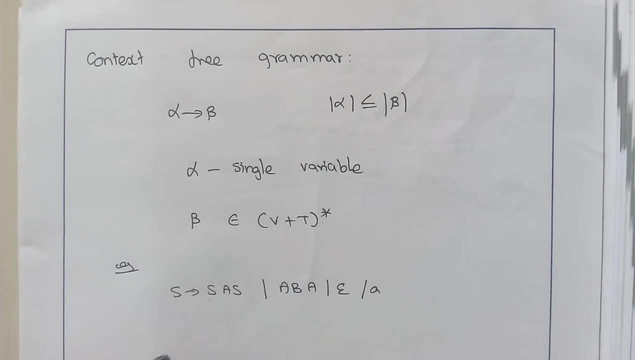 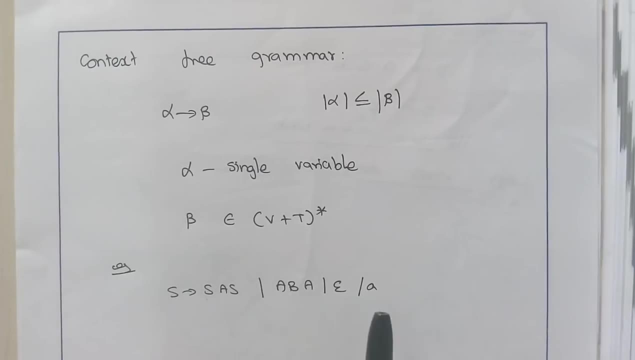 a variable and terminal. So here is an example for it: A variable, a single variable. Alpha is always a single variable that tends to any combination of variable and terminal of any length, and it also includes a single variable, So alpha is always a single variable. that 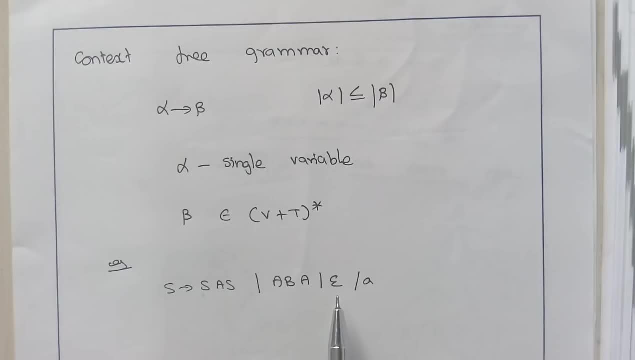 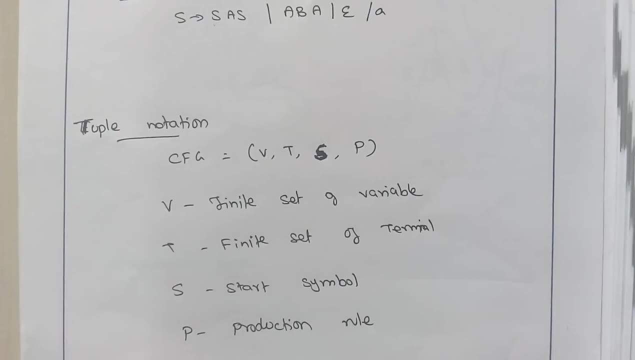 tends to any combination of variable and terminal, So there is an equation A and B in this itters. even So, a single variable can be denoted a single variable. If it is a single variable, there is an information between two rows in it, using the. 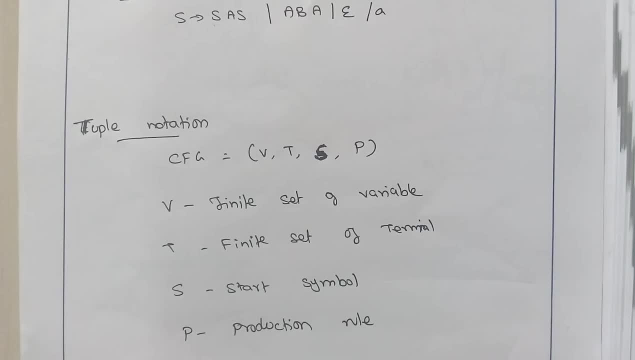 number. Whenever we are going to take some input and we are going to check whether the input belongs to the grammar or not, we have to start from the starting symbol. So S- actually it is a symbol in a variable from where the derivation starts, and P we 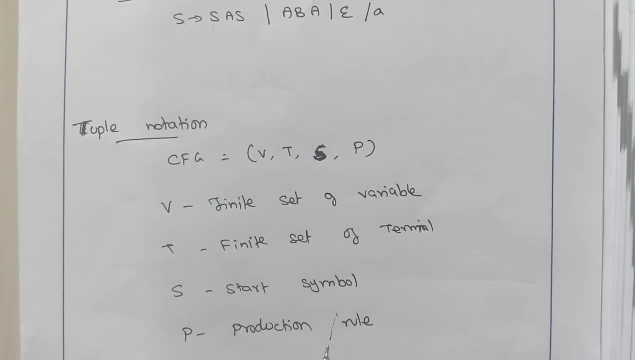 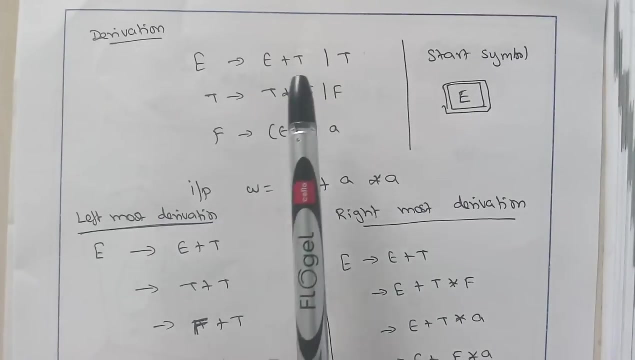 usually call it as prediction or rule, which is of the form that we have discussed previously. alpha tends to beta form it. Now we will see what a derivation is and what is a past string. Here I have taken an example for a context: free grammar. 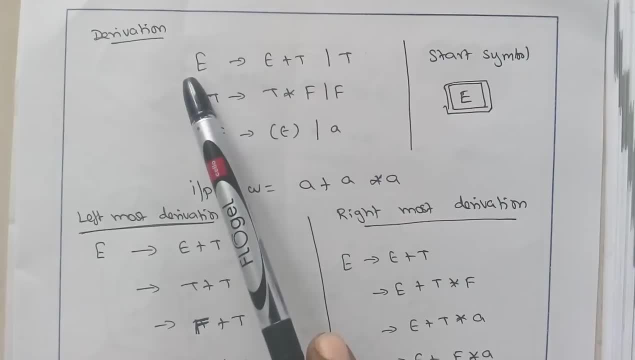 Here we have all variables, a single variable. it tends to either E tends to E plus T and when it is a slash, actually it denotes a different production: E tends to E plus T and E tends to T. that can be combined together and I write it as: 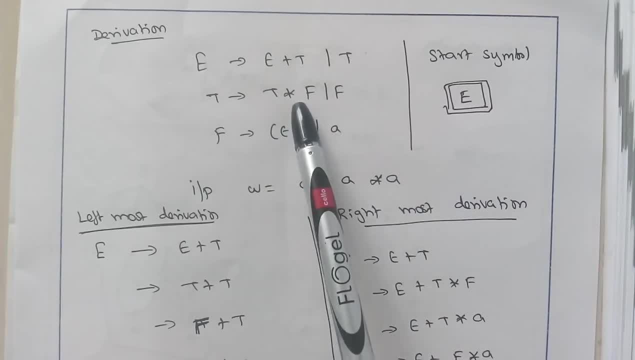 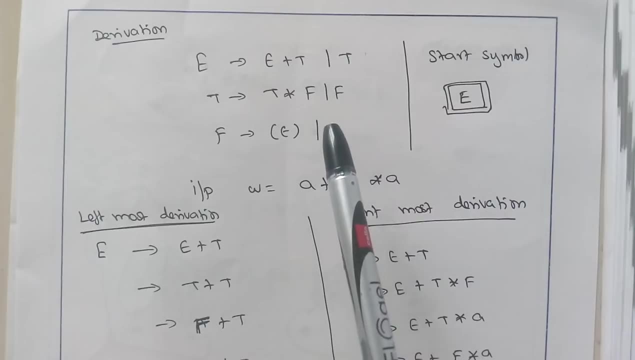 E tends to E plus T or T, Okay, And T tends to T, star, F or F, and F tends to open bracket, E, close bracket or A, Okay. So here the variable or the capital letters, that is E, T, F, for all the things, that all. 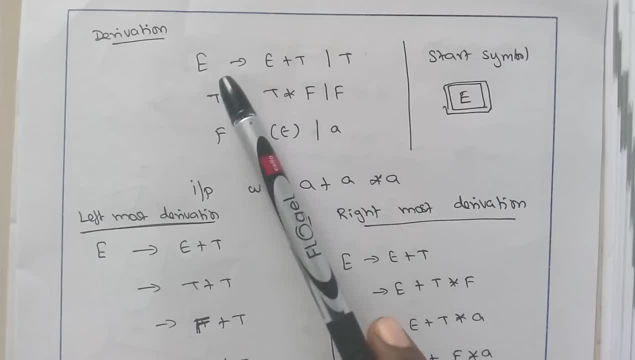 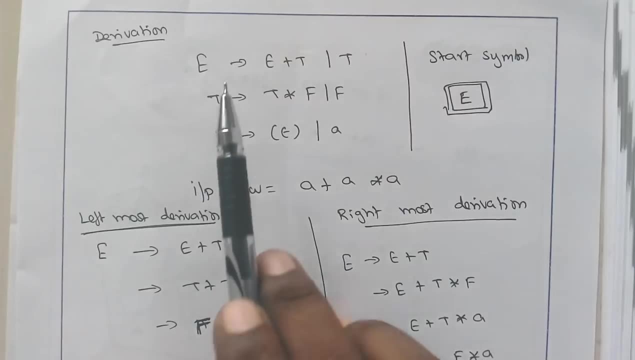 the variable it should have. we should have a derivation for it, expansion for it, Okay, For whatever is the variable that we are going to use in this context- free grammar- it should have a prediction rule for it and this terminal symbols over here. 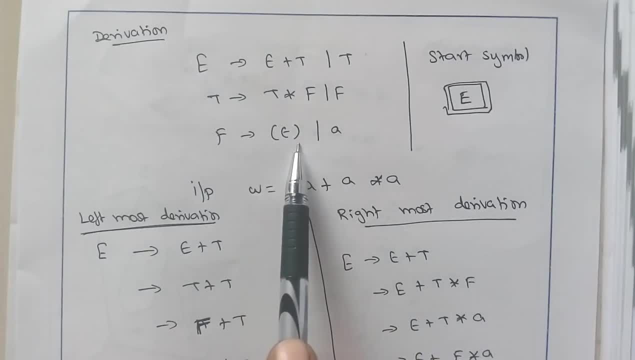 So the first one is a plus star, open and close bracket and A Whichever thing that comes in the input, the small letter, the symbols that will be included as a terminal symbol, And here the starting symbol is E. It is given that the starting symbol is E. Now we are. 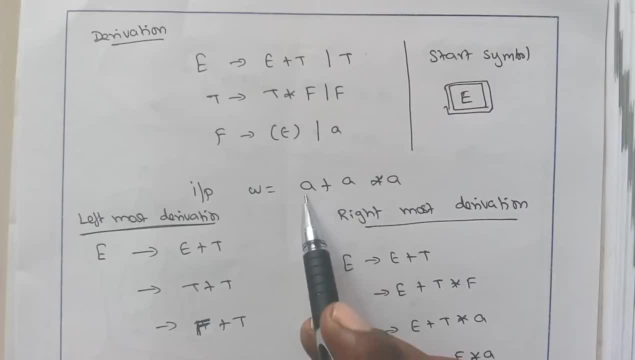 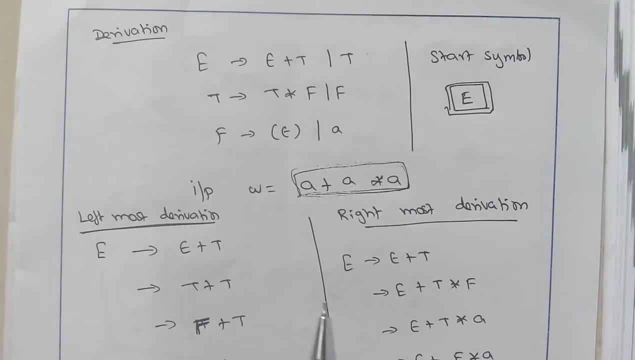 going to consider an example like input A to A- sorry A plus A star A. This is the input and we are going to check whether this input comes under this D. So we are going to check this input. It is a D in the first line. 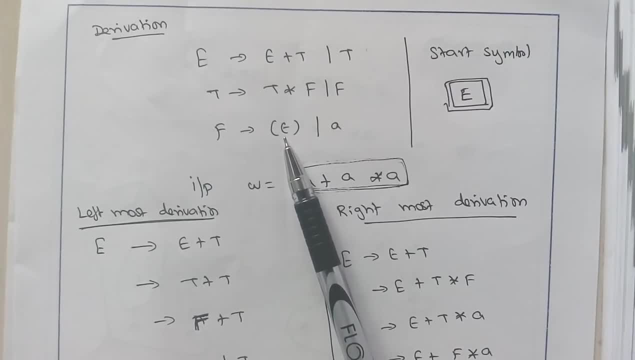 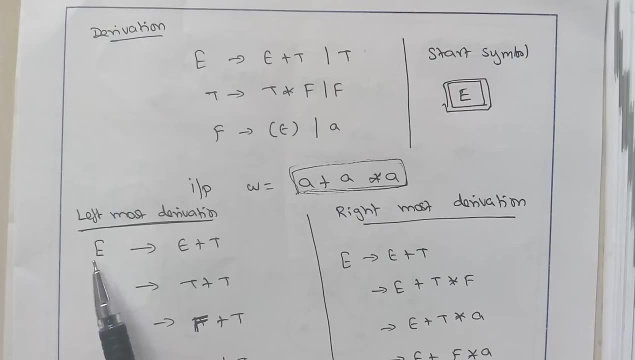 Okay, Now we are going to check whether this input comes under this A. So we want to consider grammar or not. okay, so we are going to use a derivation for it and whenever you are deriving it, we have to start from the starting symbol. so here e is the starting symbol and we can make. 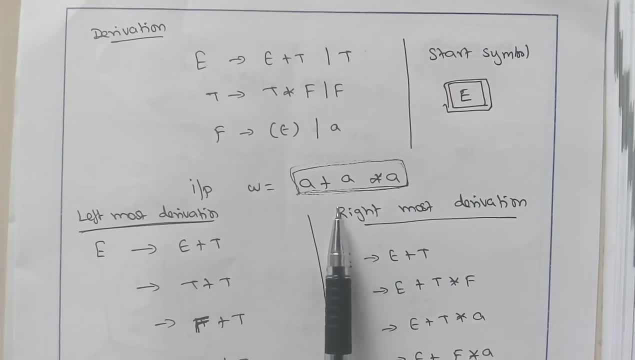 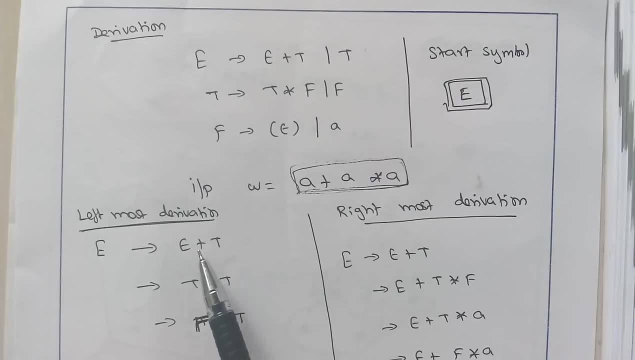 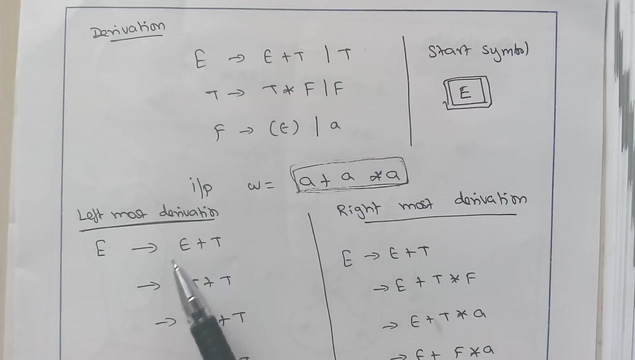 any substitution for e, but finally we have to derive this input. so first i start with: since we have a plus over here, i have taken e plus e, production, e plus t- okay, and again this e, the starting symbol should be an, a. okay, so we have to reduce this e to a. so we are going to find a way. 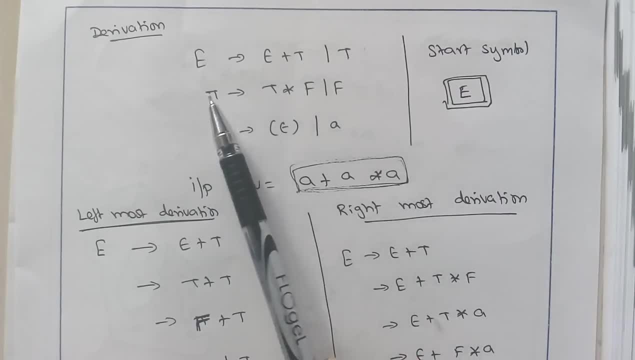 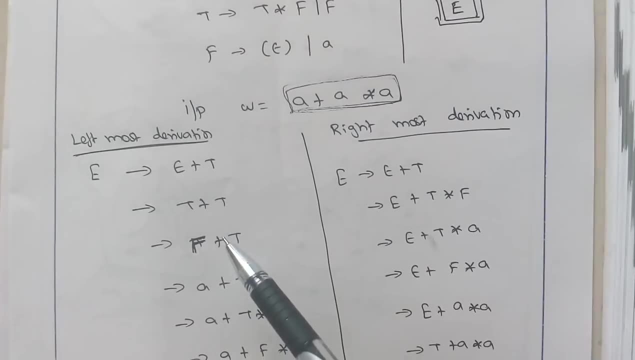 for it. so this e can be reduced with t and t to f and this f can be reduced with a. so i have reduced this e to t and t to f and then f to a. okay, so the structure will be like a plus t. okay, but our as 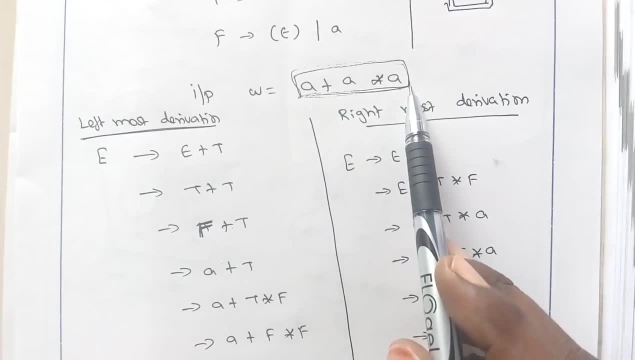 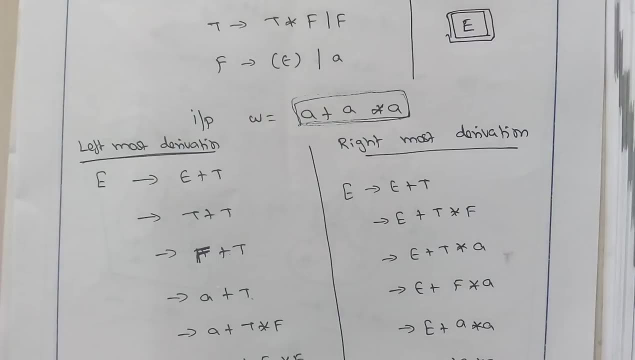 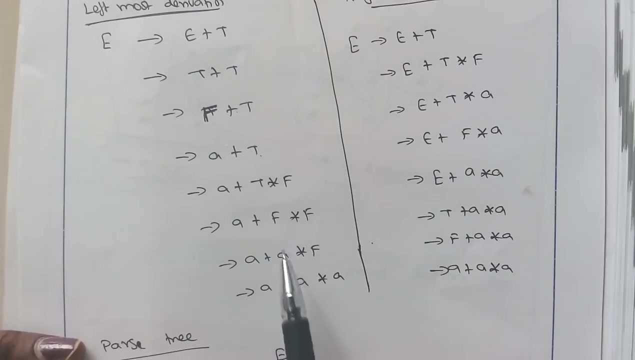 per our rule, the production should be of a plus a star a, so we need one more store operation so this t can be reproduced with t star f production. okay, so this f t is replaced with t star f and this t is replaced with f. okay, and this f with a. so this f can also be reduced with a. so finally we got the input a. 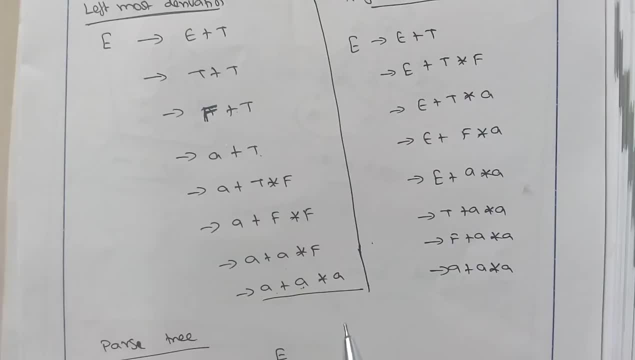 plus a star, a. okay, so this process is called derivation. for the given input, using the production that is given to us, we substitute one production at a time. for each and every variable, we substitute one production at a time and finally, we come to a derivation. we derive this input. whatever is the input given to you, we are deriving it. so this is called a. 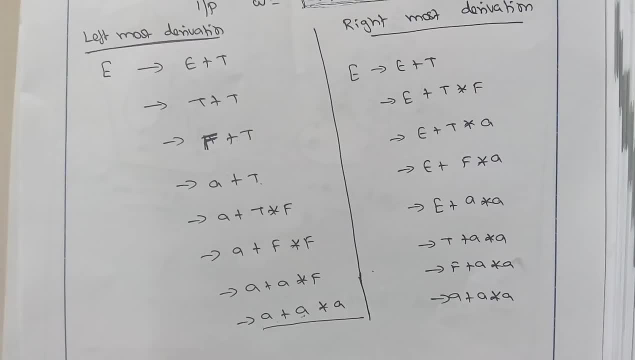 derivation, and there are two types of derivations available. one is called a leftmost derivation and another one is a rightmost derivation. a leftmost derivation is one where we are reducing this leftmost symbol first. this is a case where we have reduced this first leftmost symbol. 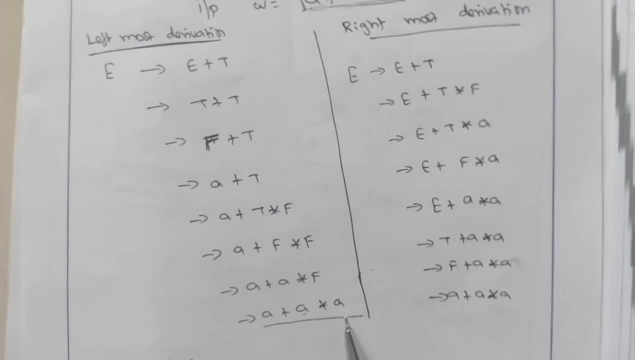 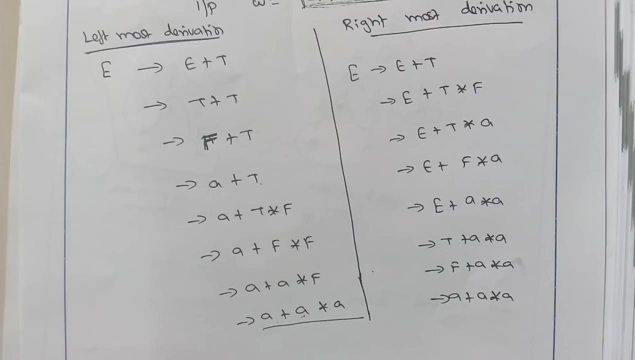 and then we proceed with the next leftmost symbol and then the last leftmost symbol. okay, so whenever are reducing the leftmost variable first, that is called a leftmost derivation, and we, correspondingly, we have a rightmost derivation where we keep on reducing all the rightmost symbol first. see this: 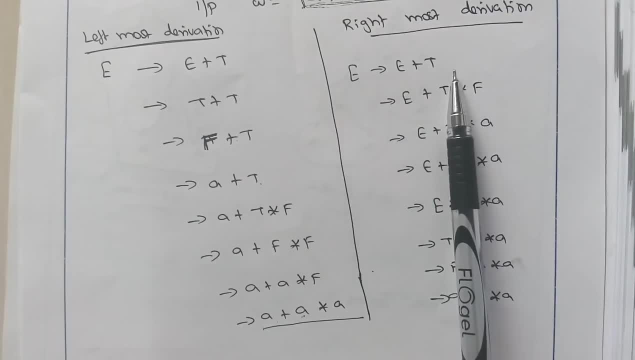 is the example for rightmost derivation you have: e tends to e plus t. i have reduced this t to t, star f first and this f to a. so i, each and every time, i just consider the leftmost variable first and i reduced it to the structure so this t can be reduced to f and f to a, and finally we come to. 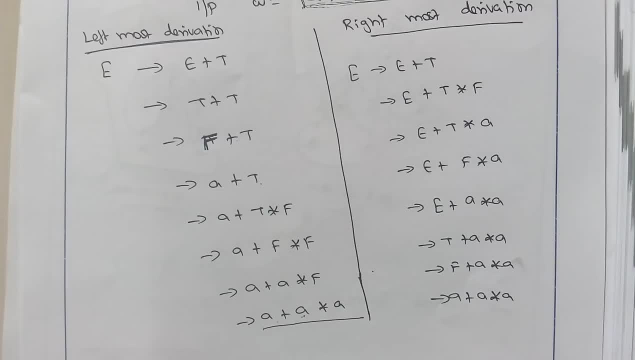 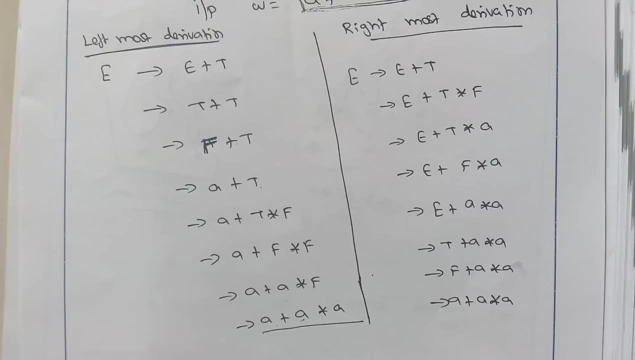 the structure e to t and t to f and f to a, so this is called a rightmost derivation. okay, each and every time we substitute one production and we derive something, so that is called a derivation. and when you make the substitution for the variable, that is leftmost. 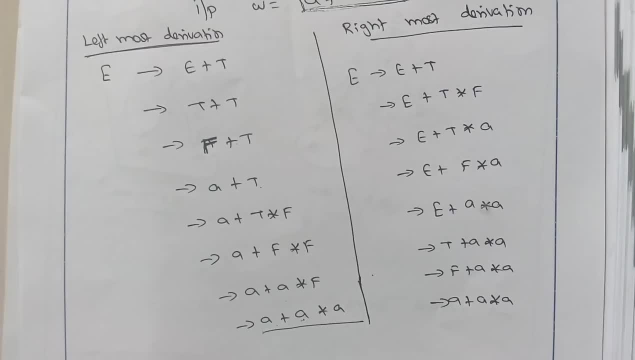 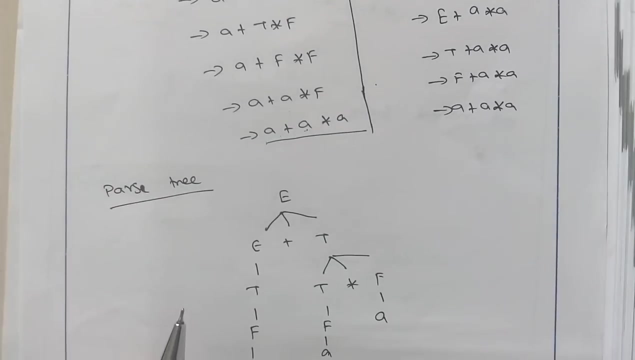 variable, first, that is called leftmost derivation. or when you keep on reducing the rightmost variable, first, that is called rightmost derivation, okay. and next, when you are representing this in a tree like structure because it as a pass-tree structure, okay. I'll give you an example for it. see here, the same. 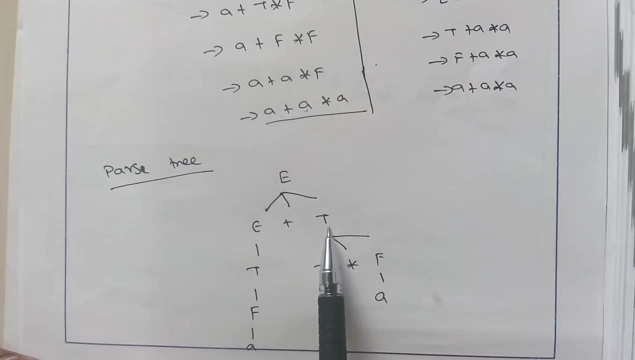 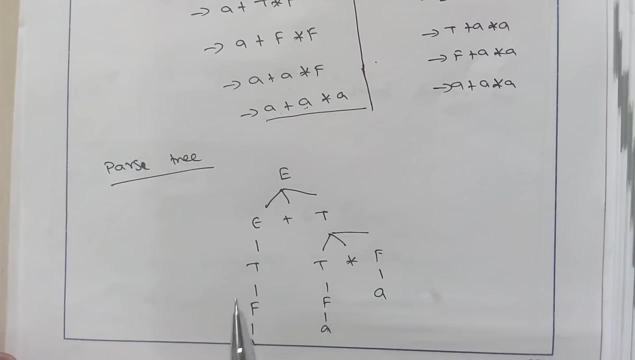 derivation. first for this E it is substituted with E plus T, and then this E is reduced to T, T to F and F to A. and here this T is reduced with T, star F, T to F and F to A and this F to A. so this tree-like structure, when the derivation is represented in a diagrammatic. 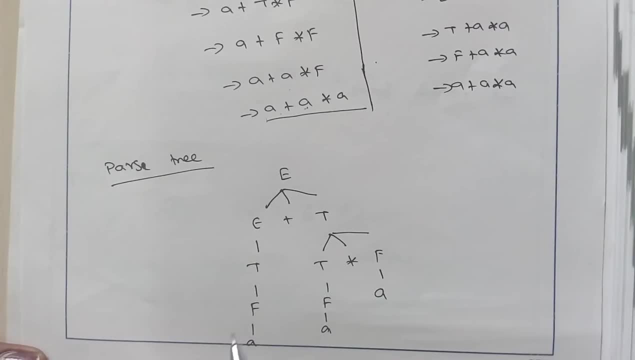 pattern, a tree-like structure. we call that as a pass-tree. okay, and while getting the input, we have to consider this leftmost branch first. okay, whatever is the leaf structure that comes in the left side, that will be considered. so it is A and this is the leftmost. 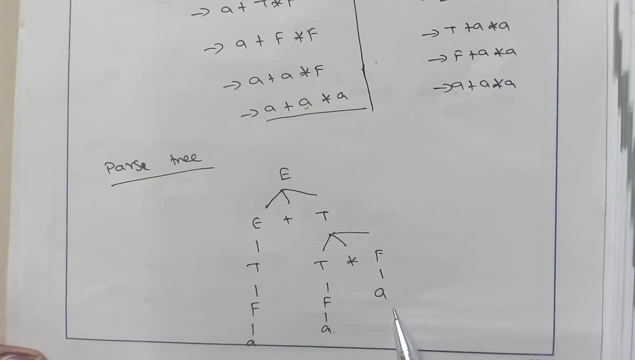 symbol: A plus A star, A. okay, we are going to consider all the leaves altogether to derive the input. okay, and we have to consume it from this leftmost side. so A plus A star, A, okay. so this is called a pass-tree structure. 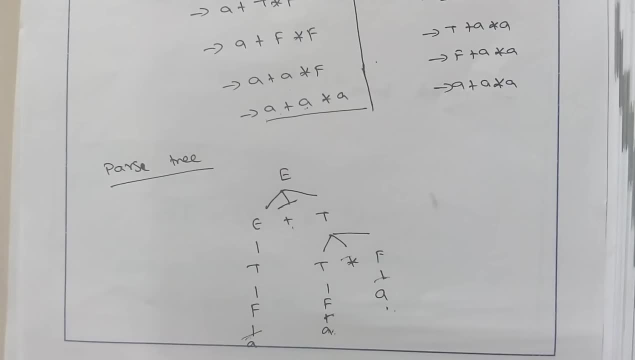 And there is one more. There is one more condition, like for the same grammar, for the same input, if there is a possibility of deriving to R more pass-tree, we call that problem as an ambiguity problem. okay, we will see an example in that. 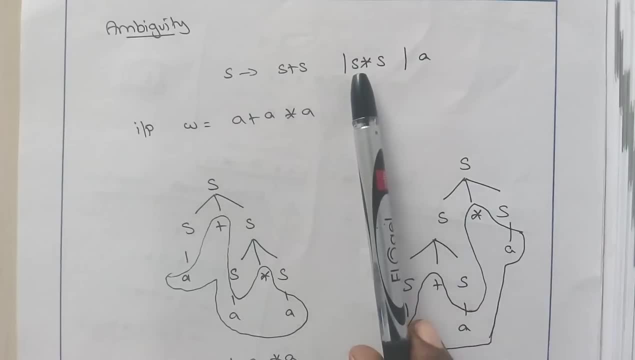 Consider this case. we have S tends to S plus T S star S. sorry, S plus S or S star, S or A. okay, so S has three different rule for it. one is S plus S, another one is S star. 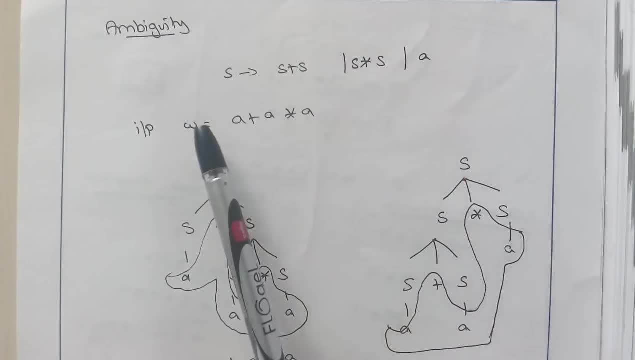 S and next one is S tends to A, and we are going to derive the input A plus A star A. okay, so here I need A plus A star A. so first I either take S plus S or S star A, S. okay. 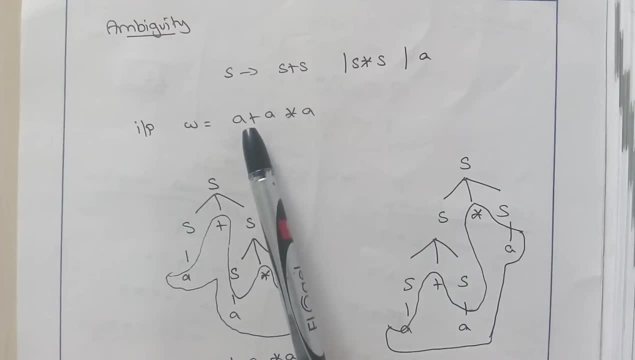 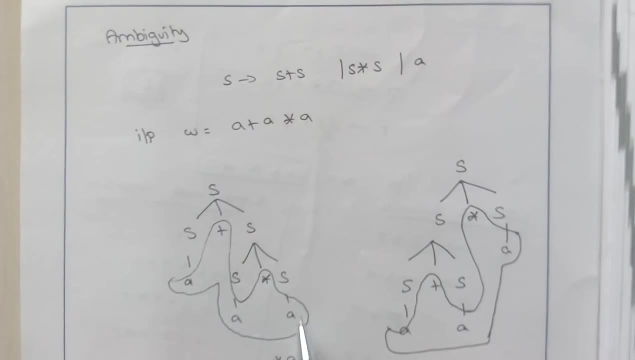 so, in case, if I am taking S plus S first, okay, so this plus is over here, so this S can be reduced to S star S and, finally, each and every S can be substituted with A. this is one way of deriving it, and here is another way of deriving it. 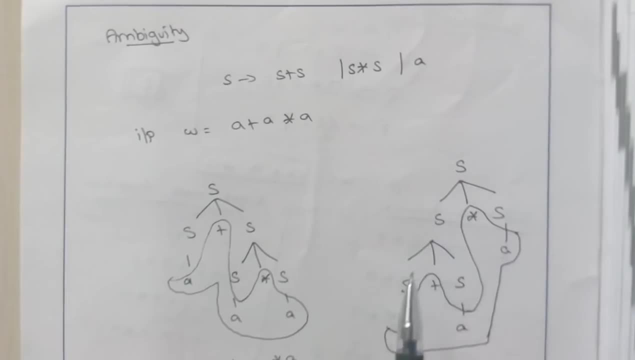 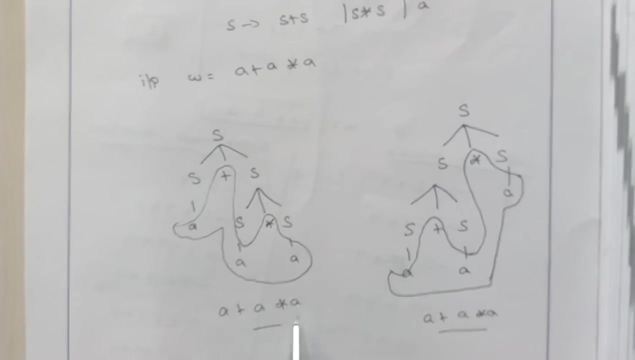 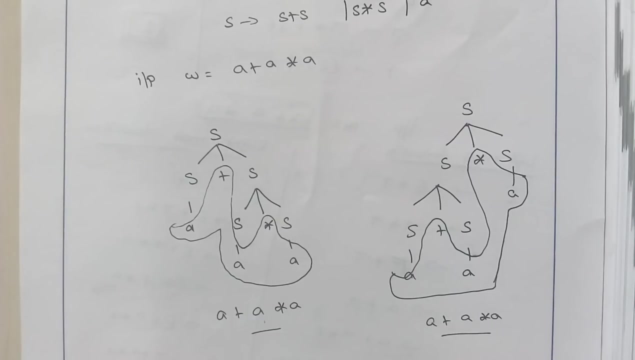 I start with S, star S first, and again this S. I am substituting S plus S. okay, but still I derive to the same input: A star A plus A star A and A plus A star A. okay, so for the same grammar, if that, and for the same input if there exist two R more different. 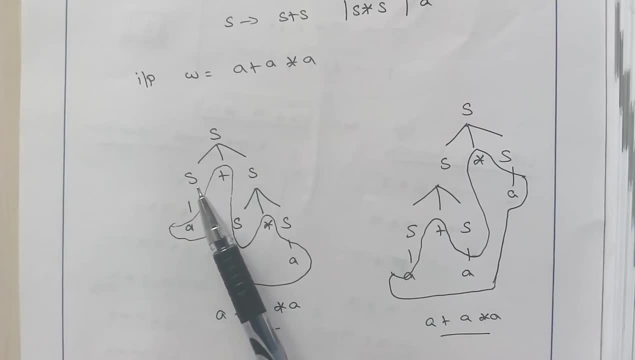 pass-trees. see, the structure is different. see, here I have taken S plus S first and here it is S star A. okay, so totally, the derivation is totally different. okay, So when these type of structure exists, we call that as a ambiguity condition and we